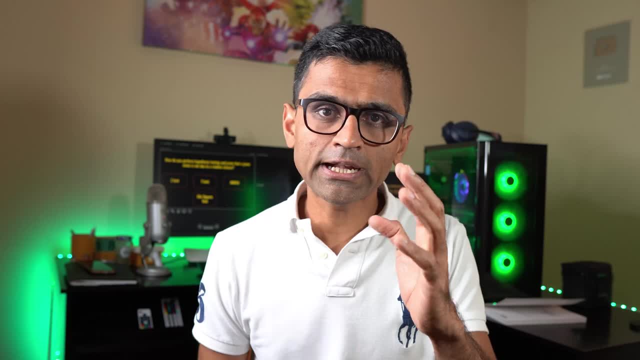 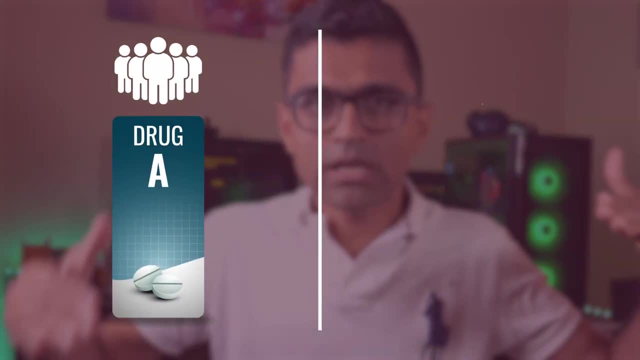 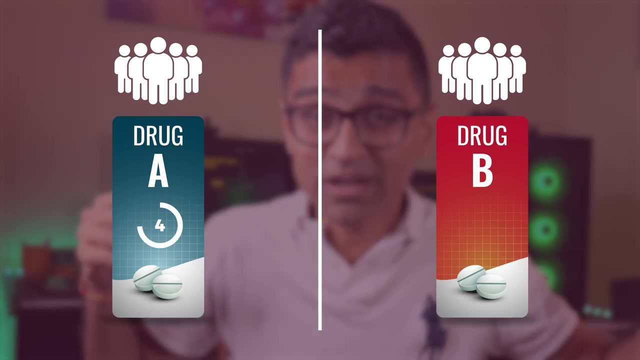 do a clinical trial. How about you get ten volunteers and ten volunteers who are having headache and give drug A to five volunteer and drug B to remaining five and kind of measure a time. Let's say drug A takes four hours to get rid of headache, drug B takes only three hours to get rid of headache, Did we? 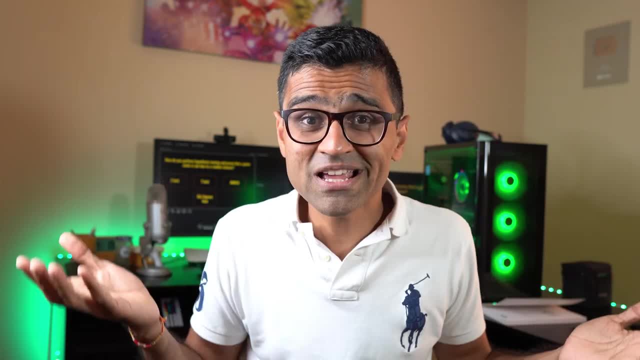 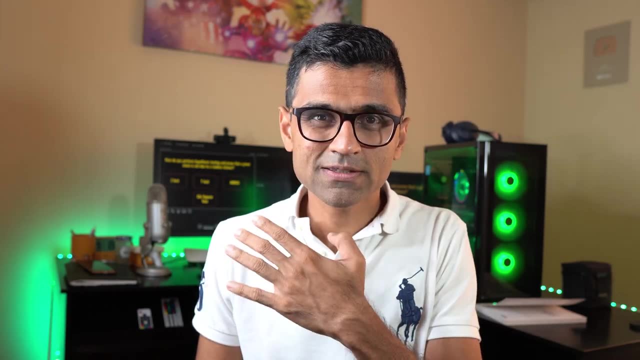 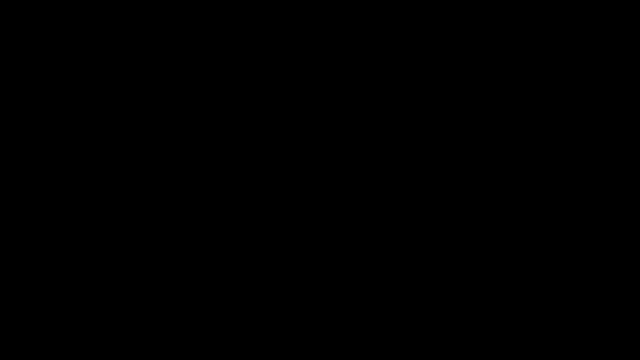 prove that drug B is effective than A? Well, obviously answer is no, because our sample size is very small. Instantly, since you can't taste certain things on the entire population, we take a sample and hear: our sample was ten volunteers, and ten volunteers versus millions of. 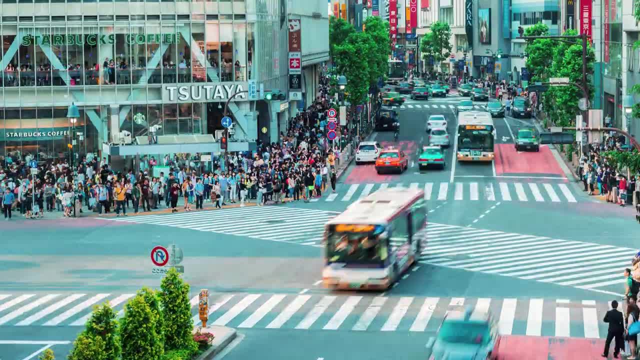 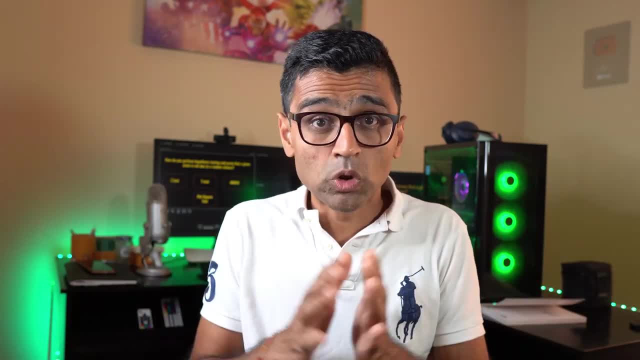 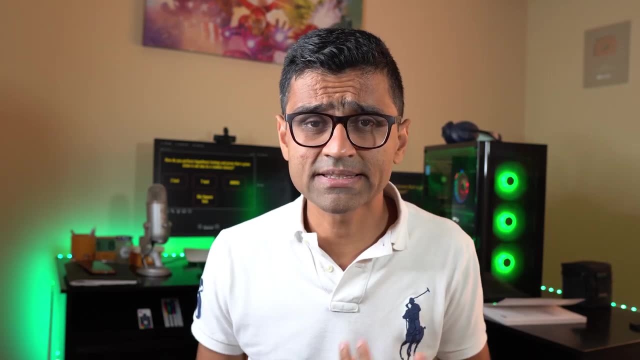 people is definitely a very small sample. So we can say that maybe this happened because of a random chance, or the sample is not good enough to give you confidence that B is more effective than A. Then what do you do? Well, we can increase the sample size. Let's say you take a. 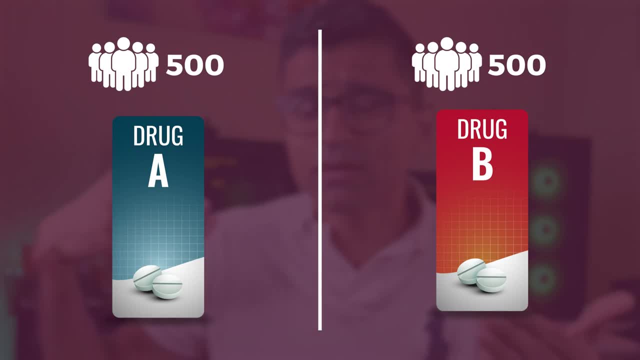 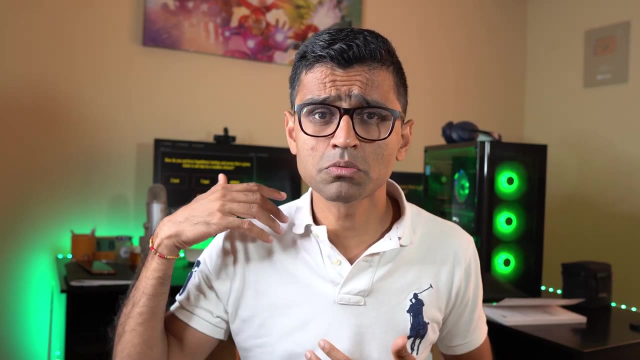 volunteers- maybe 500 are taking drug a. 500 are taking drug b. again, drug b takes average three hours. the drug a takes average four hours to get rid of headache completely. have we proven that b is effective and are we in a position to roll it out to millions of people? well, maybe not, not. 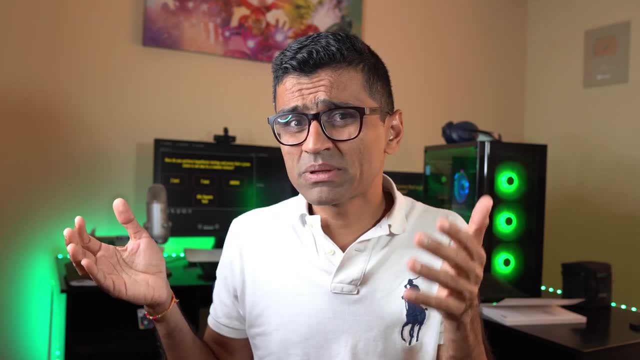 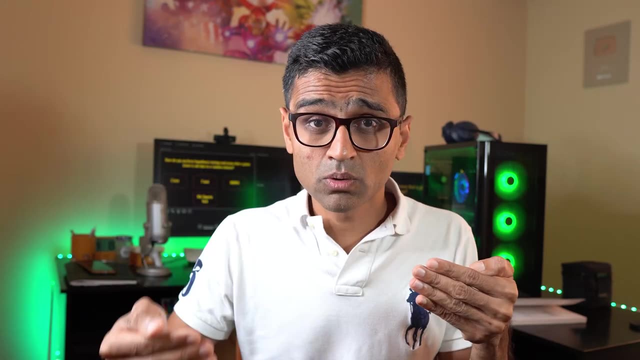 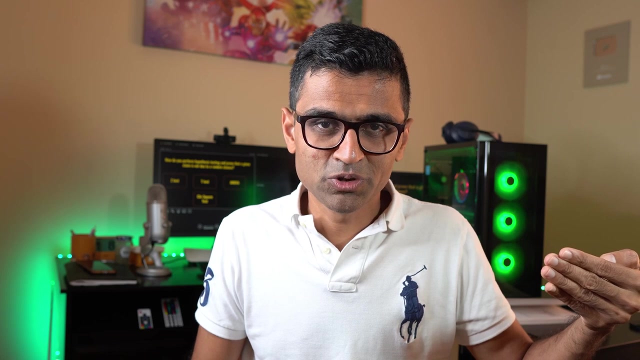 sure, because thousand versus millions of people, maybe thousand still is not a big enough size. other problem is: what if the 500 people on whom you tested b are all young folks you know with better immunity, and remaining 500 people on whom you use drug a they are old folks or they have? 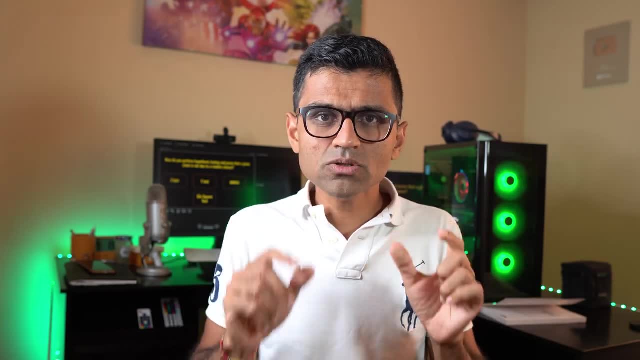 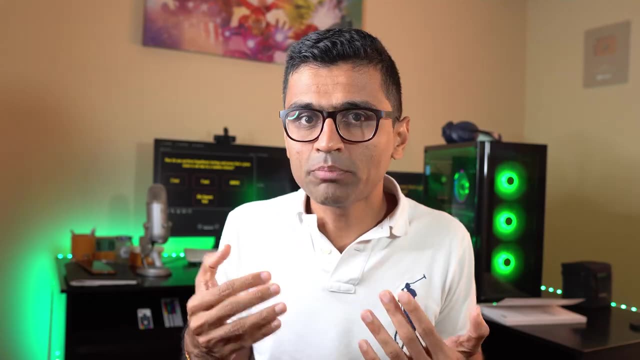 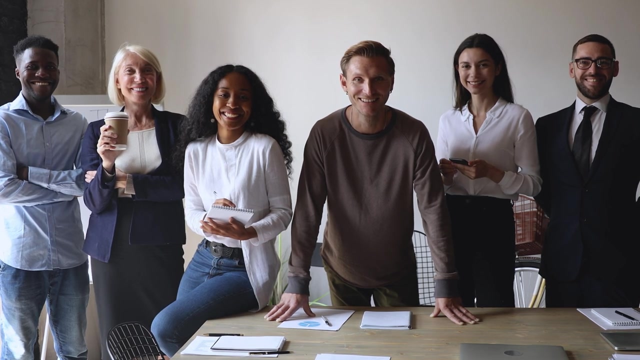 underlying condition. their immunity is little weak, you know. so it depends on the two factors. one is the sample size and how much variation you have in that sample. do you have people from all age groups, different medical condition, different ethnicity? you need to consider a lot of factor in order to conduct an effective 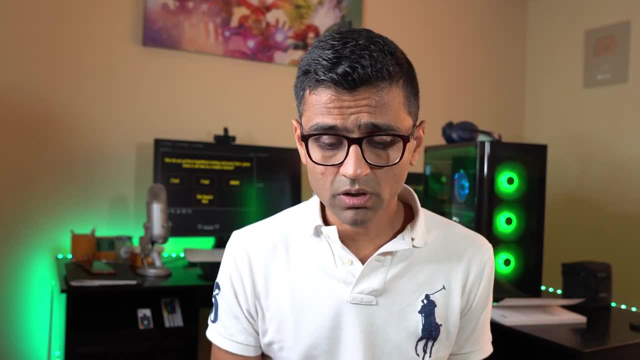 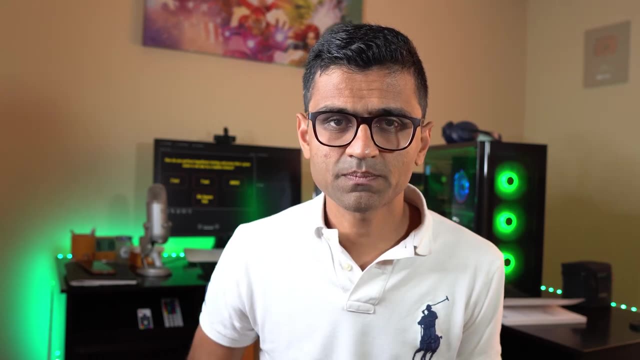 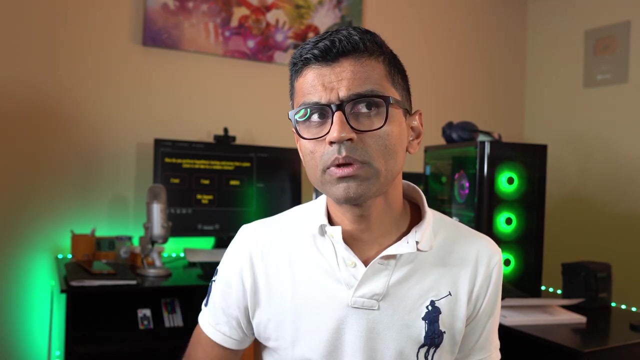 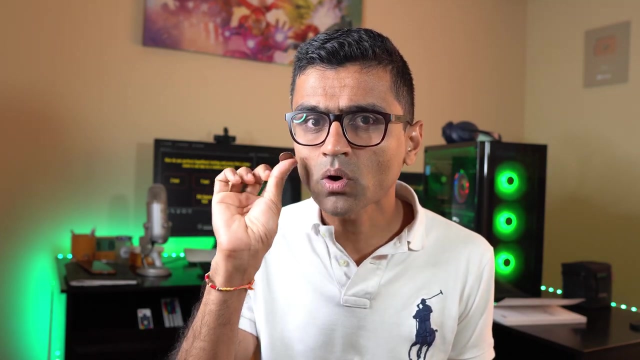 test. now let me give you another example of coin flipping. so what I did once is I had this coin, I flipped it seven times and usually you expect that you will get head and tail. you know equal number of times. what happened for me is in first four times I got head and I started thinking maybe there is something wrong. 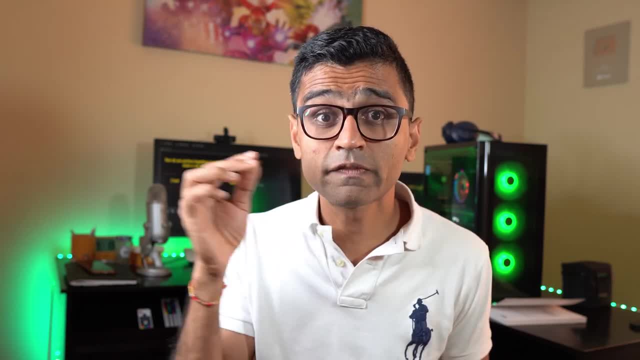 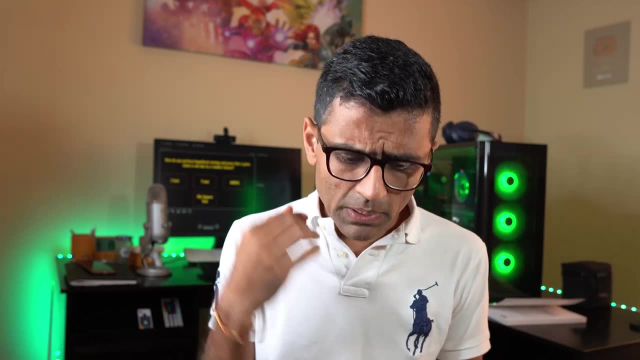 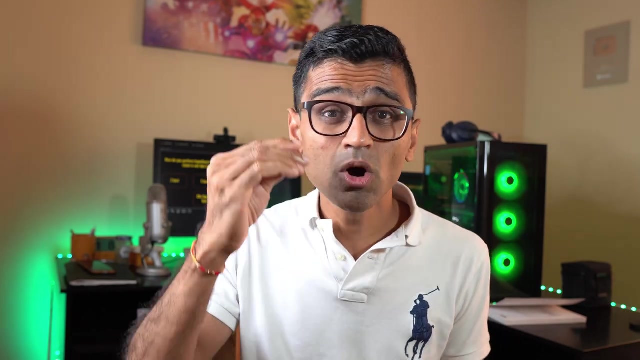 with this coin. maybe it's counterfeit, maybe it is favoring head. so you can try this experiment. try flipping this coin so many times and many times. you will find that you know, four times, five times, even six, seven times in a sequence you might get head or tail and you will think there is something wrong with the. 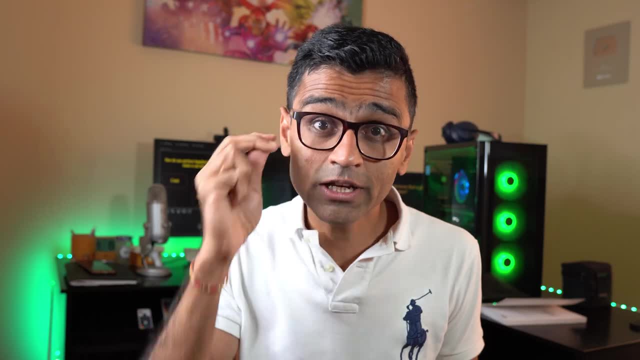 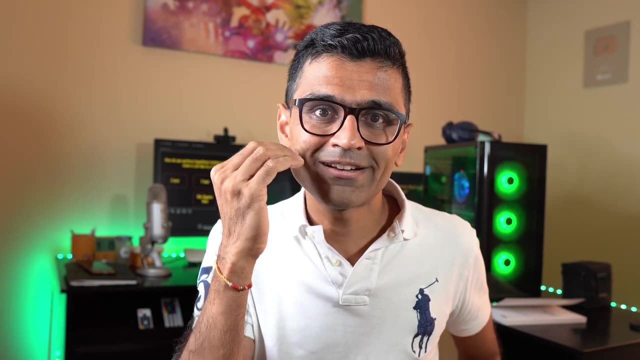 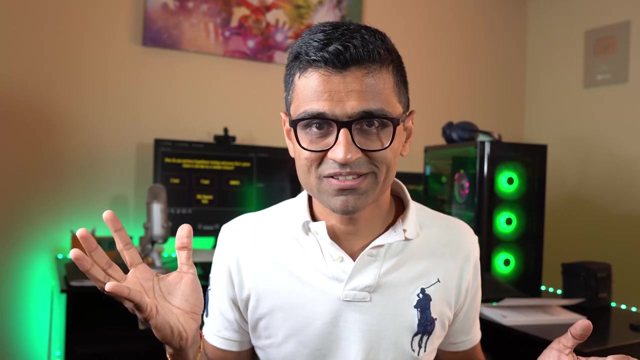 coin, but the reality is that nature tricks you. nature tricks you in a way that you will start thinking that there is an underlying reason behind an event or a phenomena, whereas the fact is that it is pure randomness. this is the natural law. I am from India. I have seen. 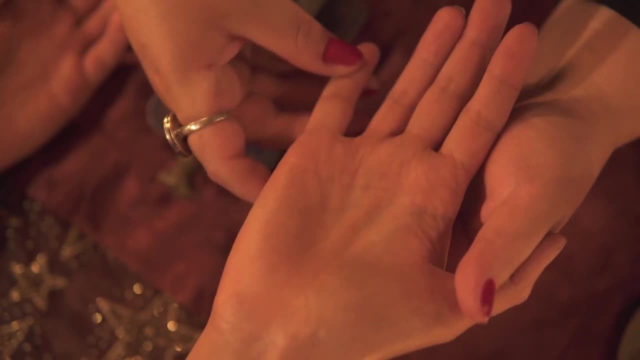 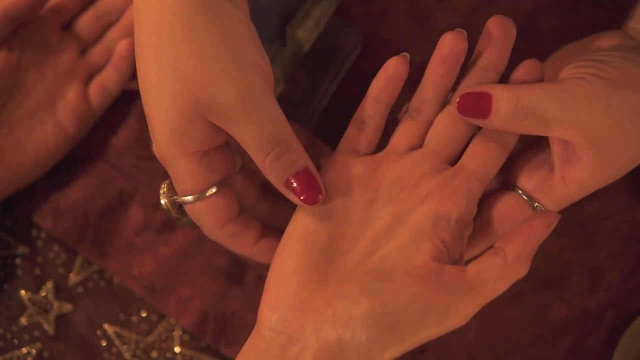 enough examples of successful astrologist who try to predict your future. who will you know that there was one astrologist who used to say: you know that there was one astrologist who used to say: you know that there was one astrologist who used to say: 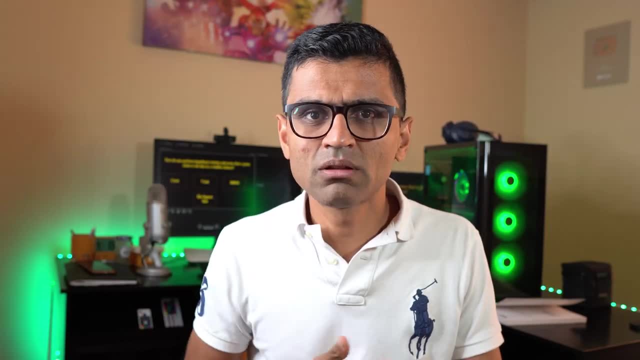 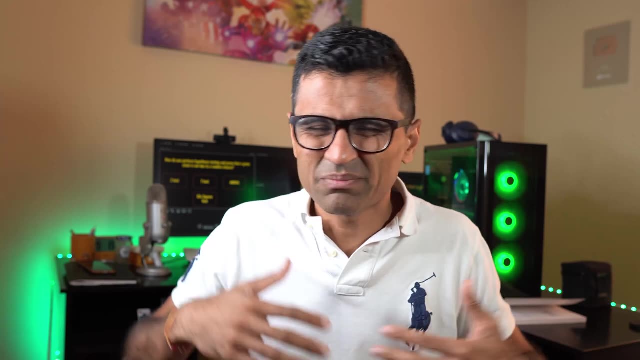 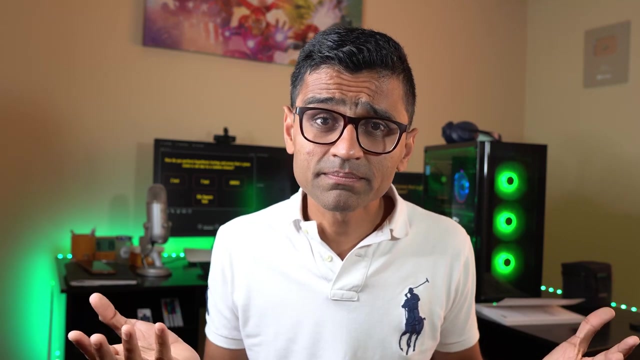 that okay, at age 35 you will. you will have unexpected monetary benefit. maybe you will win a lottery or you will get a prom like bonus or something. now, if you make that claim- 200 people, maybe 20 or 30 people- you will get it right and 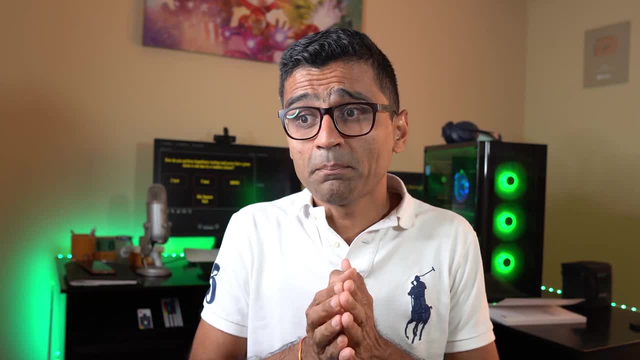 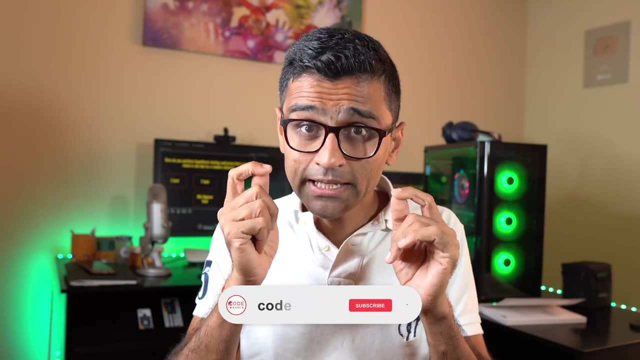 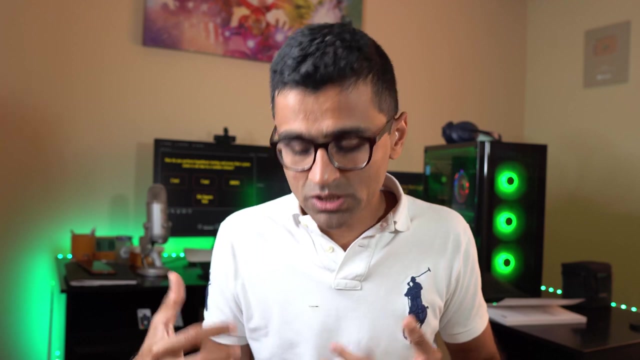 that's just because of pure randomness. but then people think that no, this astrologer knows how to see the future. so they they think of randomness. you know, actually, the underlying causes: randomness, but the way the events are happening in nature it makes you think that there is an underlying reason and 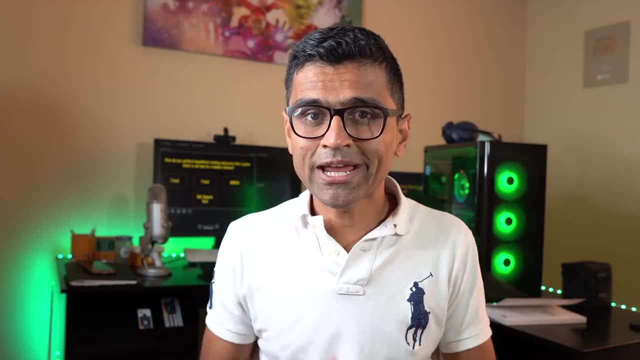 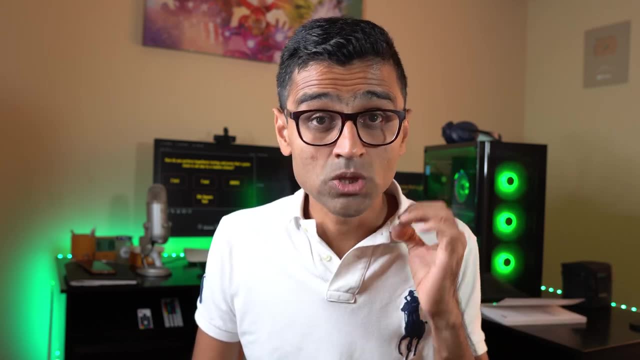 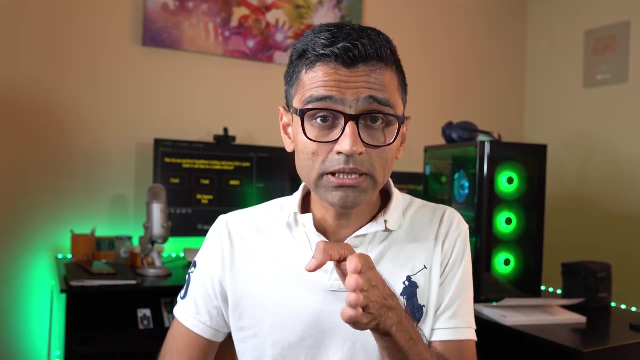 the purpose of hypothesis testing is to get rid of this element of randomness. basically, it is to figure out that observed result is not because of a random chance and there is a strong reason behind it. so in our case, drug B is more effective than a, and in our case, drug B is more effective than a. and in our 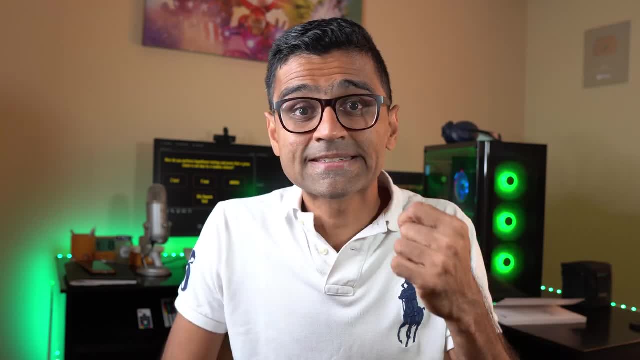 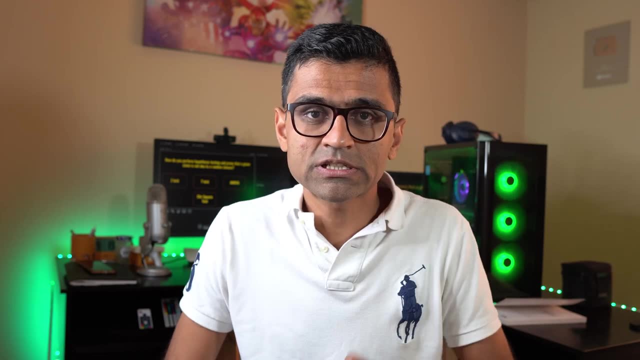 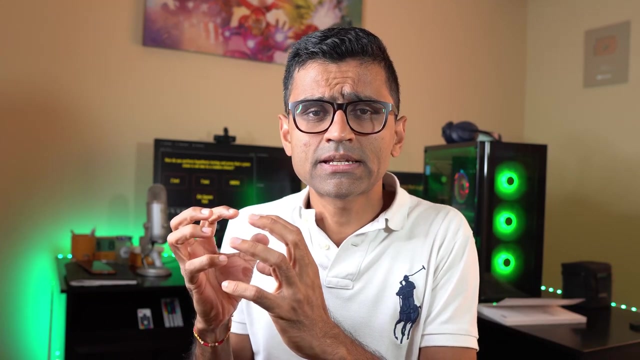 case, drug B is more effective than a and in our case, drug B is more effective than a. hypothesis testing allows you to rule out the element of a randomness. so if you do hypothesis testing, you can scientifically prove that drug B is more effective than a. and how exactly hypothesis testing is conducted is: 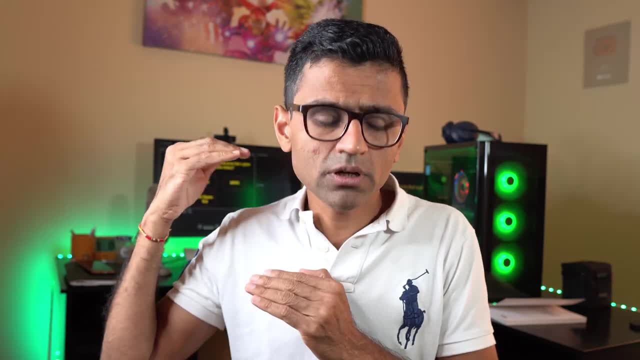 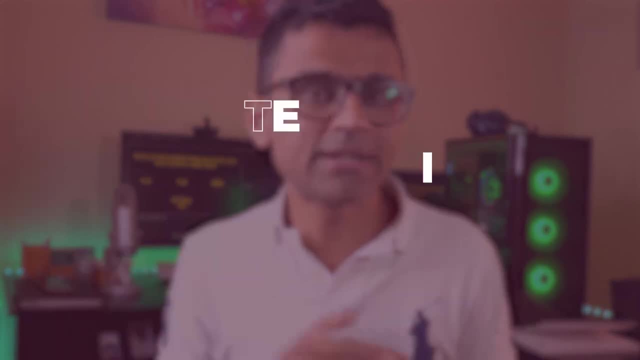 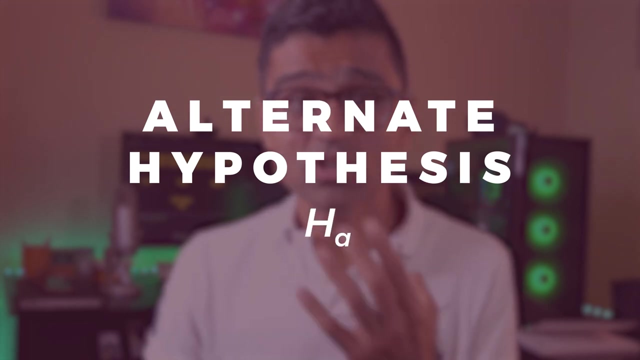 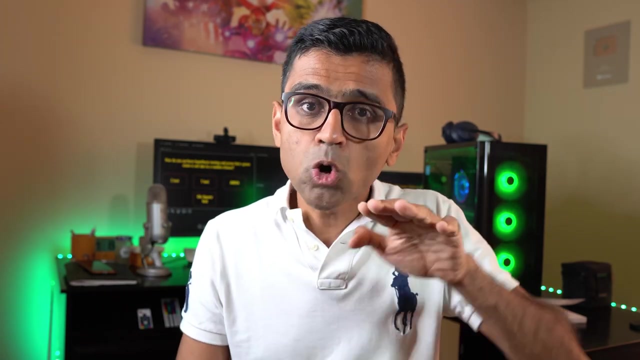 beyond the scope of this video, but I will talk about some of the methods now. in our case, drug B being more effective than drug a is called alternative, alternate hypothesis. An alternative hypothesis is, you know, represented using HA. So HA means the claim you want to prove, and we always come up with the opposite hypothesis, which is also called a. 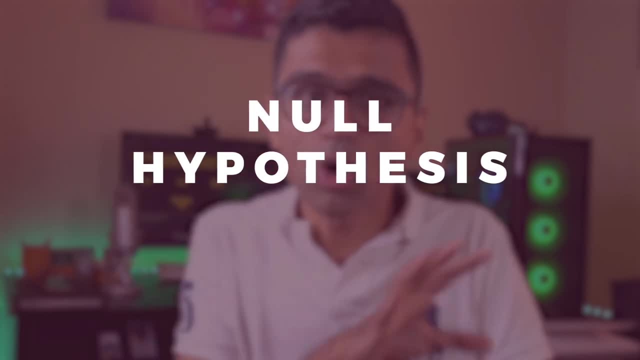 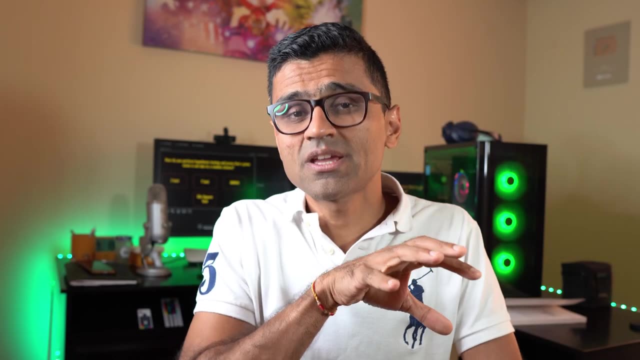 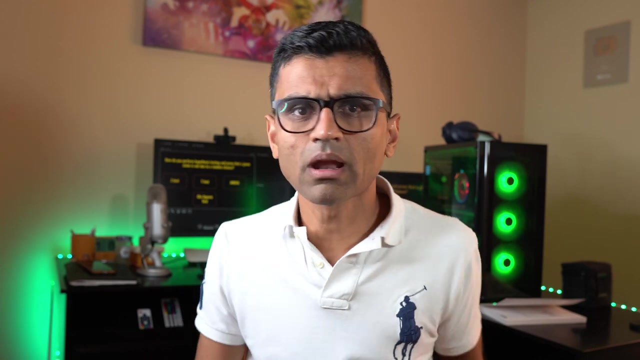 null hypothesis, which is: drug B is not more effective than drug A. So drug B not being more effective than drug A is null hypothesis. and null hypothesis and alternate hypothesis. they are exactly opposite. Now why do we need null hypothesis? Why can't we directly prove that? 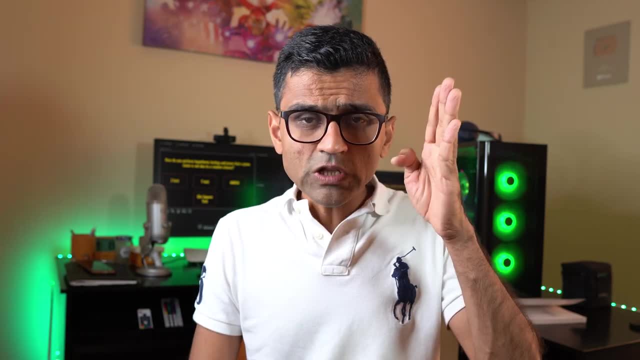 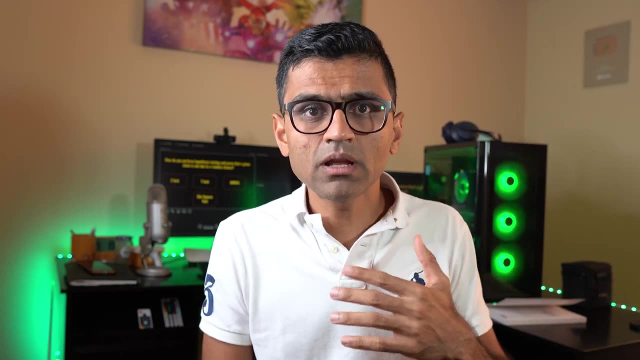 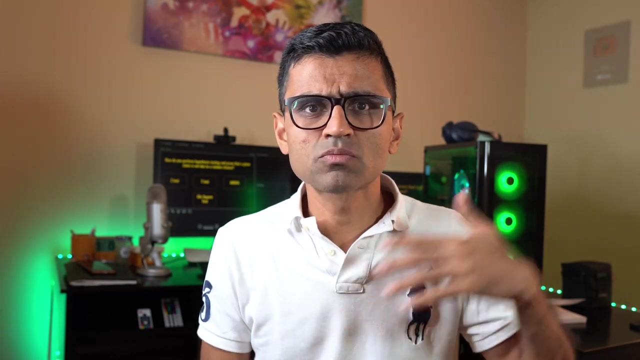 drug B is more effective than drug A. Well, null hypothesis, first of all, represents the established fact. What is the established fact? Well, drug A is the most effective drug by pharmaceutical in the market. So drug A has been used by millions of people since past five years, and it is the established. 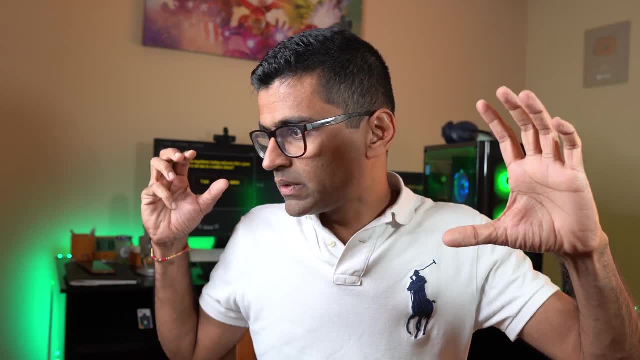 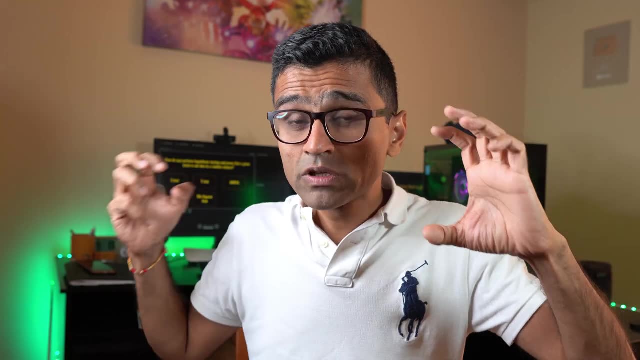 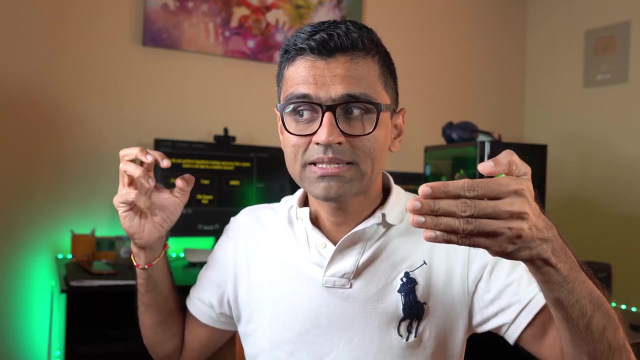 fact. and if someone is coming up with drug B and saying that, okay, drug B is more effective, we want to play devil's advocate. We want to look at that claim with a lot of skepticism and start our inquiry by saying that no, drug B is not more effective than drug A. 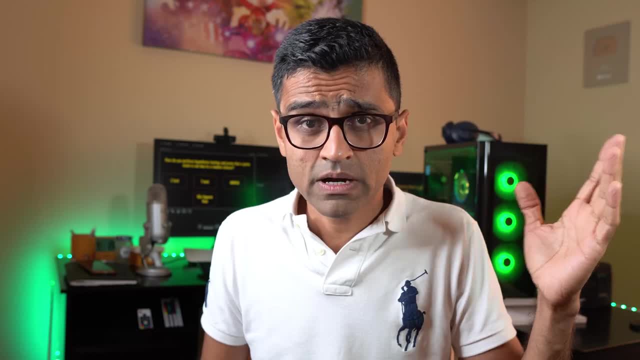 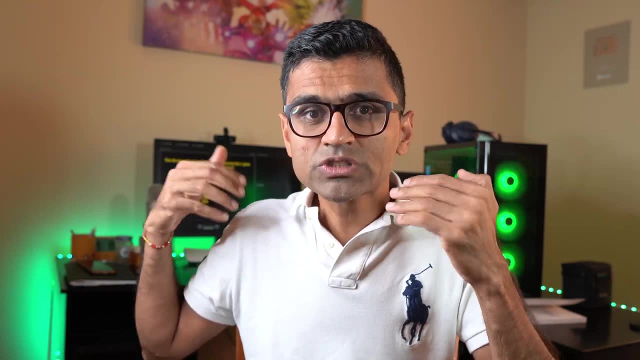 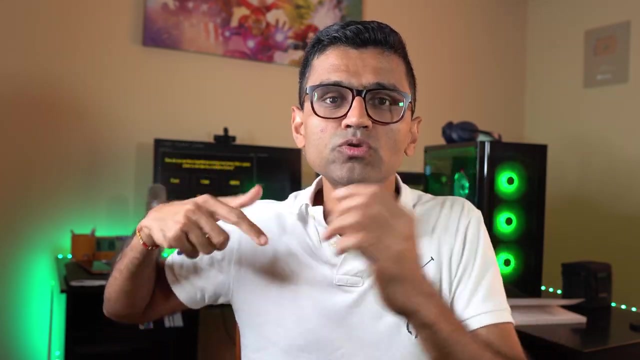 Drug A has been very effective Since past five years. so many people have used it. so I don't believe drug B is more effective than A. So we want to start with the established fact, you know, whatever is true as of now, and then we do couple of tests, you know, using hypothesis testing, and try to prove that. my null hypothesis. 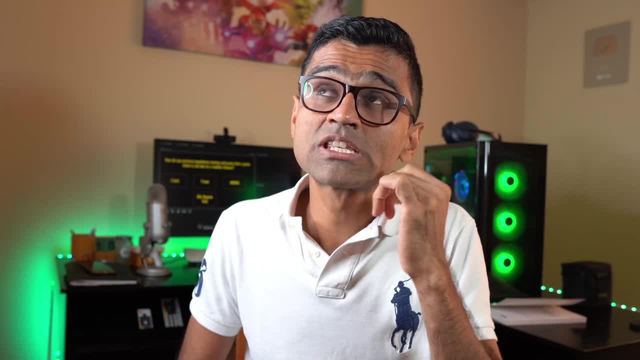 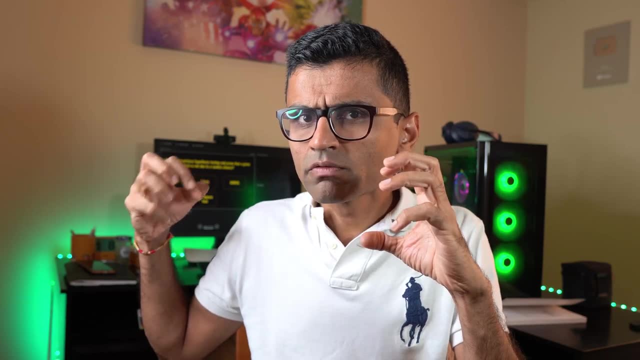 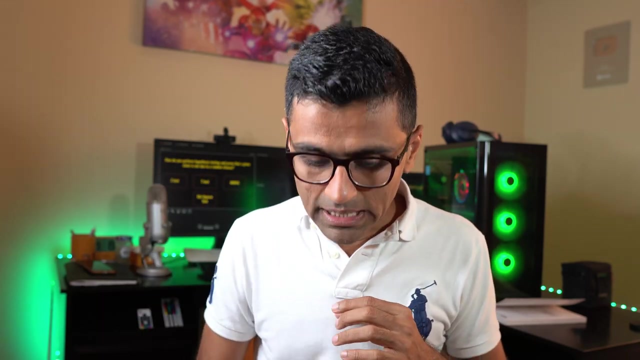 is wrong or my null. we try to reject the null hypothesis. basically, We try to reject that drug B is not more effective than A. When you reject that, you automatically prove that drug B is actually effective than drug A. It is like going to a courtroom. you know, someone committed. 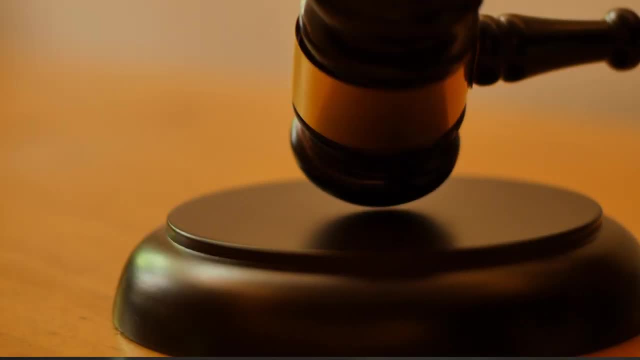 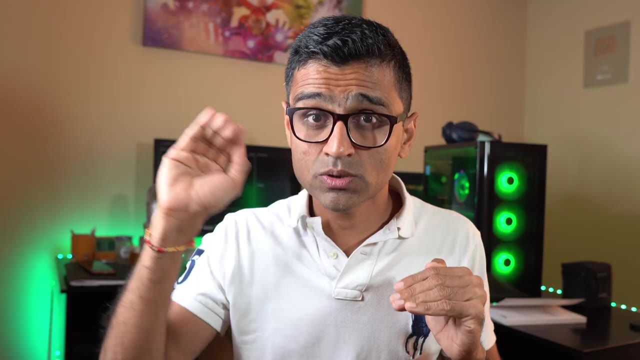 a murder, but we always say innocent until proven guilty. So in the court we will always start with us by saying that, okay, this person is innocent, They have not committed a murder and DIY 😊ging8. 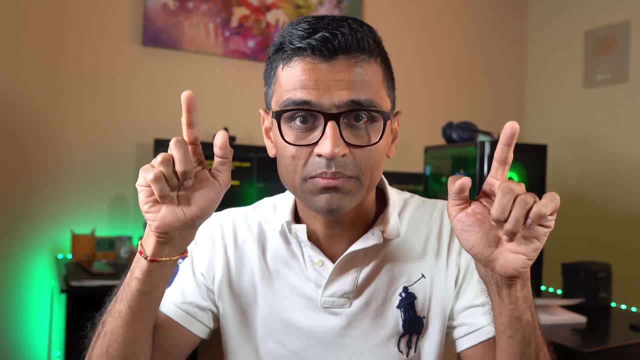 To dad: do not commit a murder and then you need to employ Jesuitism was instead of an will. try to reject that statement. So null hypothesis is: the person is not guilty and the 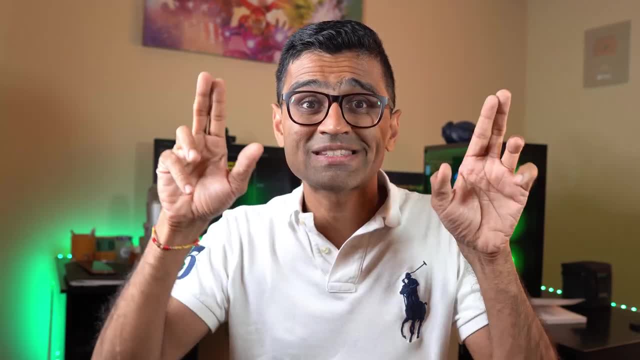 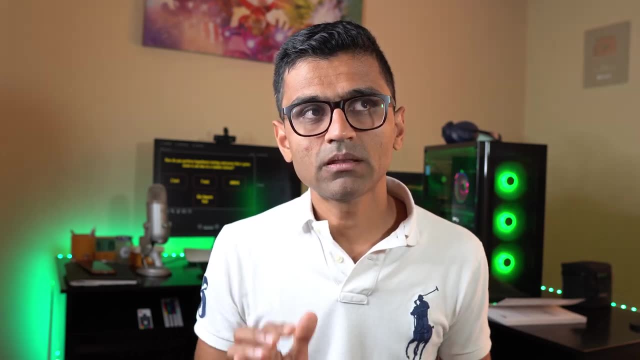 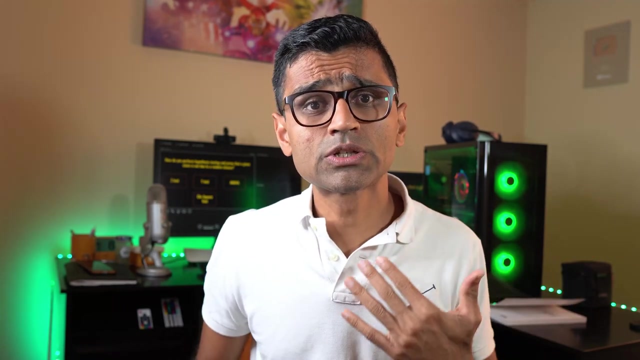 lawyers on the opposite side will try to prove that this statement that the person is not guilty is wrong, and by doing that they prove that the person is guilty. There are many examples of null hypothesis and alternative hypothesis and I'll go through some of them Back in time. it. 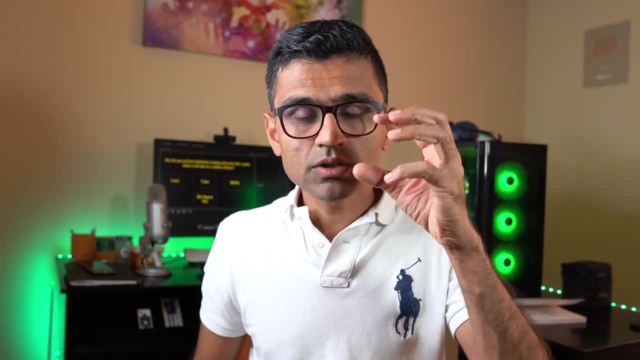 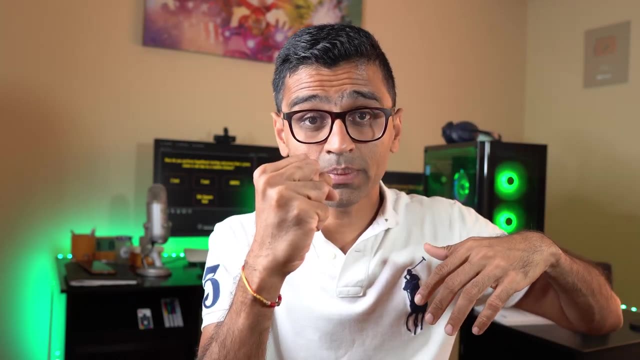 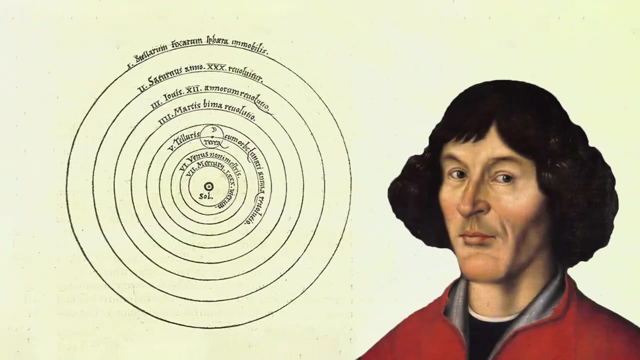 used to believe. people used to believe that the sun rotates around the earth. So people in back in days used to believe earth is static at the place. sun rotates around it. Then Copernicus came in with a theory that no, that is not true. So the null hypothesis at that time was: sun rotates around. 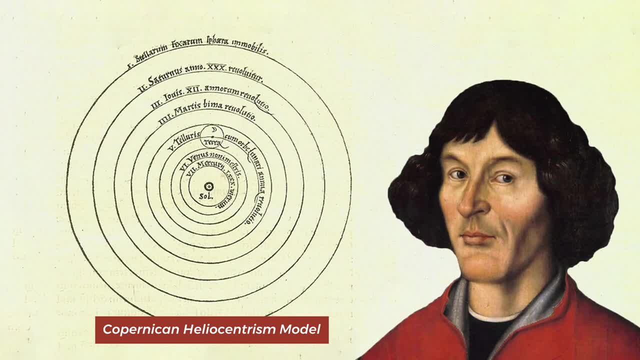 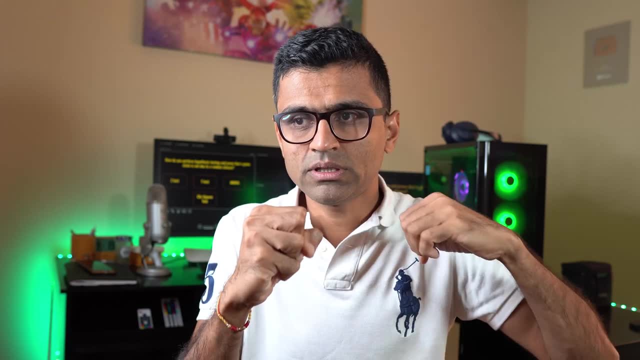 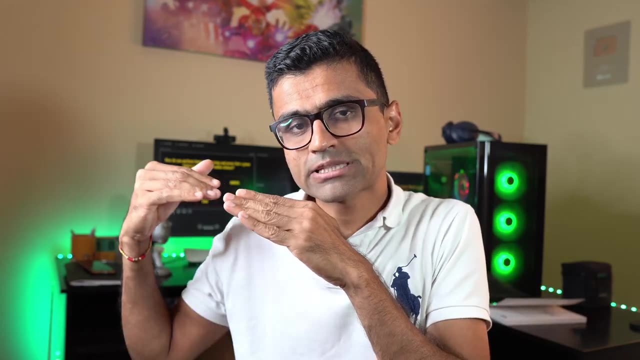 the earth. It was a widely accepted belief for many years. and then someone comes and says that no, This is not true, that sun rotates around the earth. and when you reject that claim, automatically the second most claim that is there becomes kind of an established truth. So the way it works is: 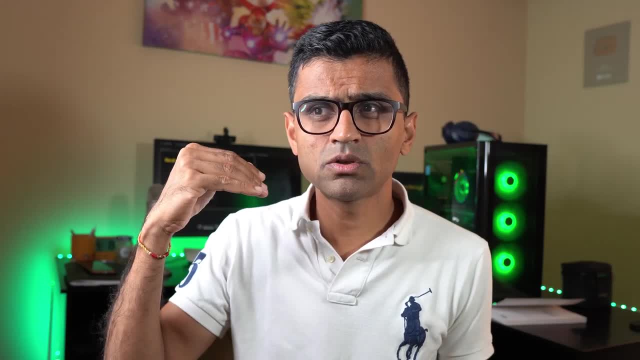 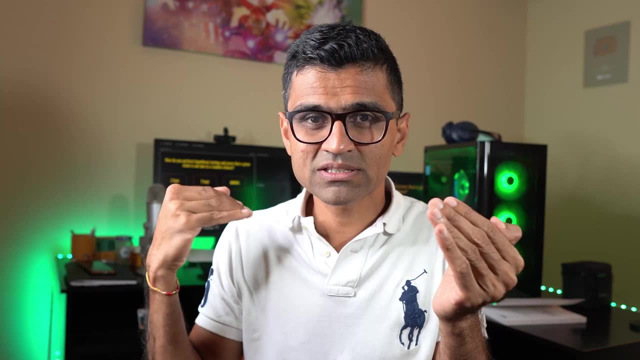 the claim that you're trying to prove. you cannot say for sure that this is the truth. So, whatever is the opposite, you try to reject it and then this second most established thing kind of becomes the truth. So the way it works is that the claim that you're trying to prove 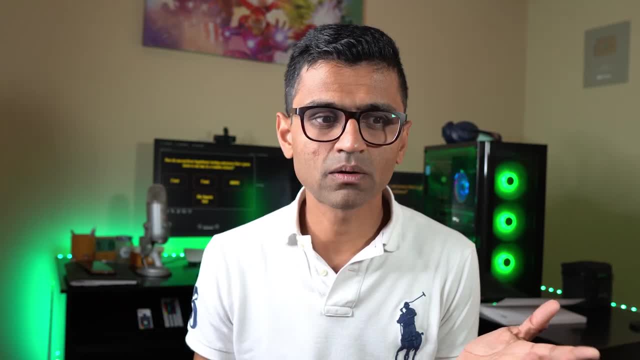 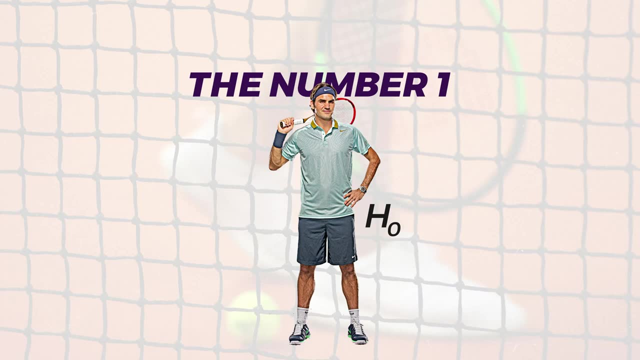 yourself wrong becomes the truth. It's like you know, at some point Roger Federer was number one player one one number one tennis player. So the null hypothesis is: Roger Federer is the best tennis player. Then Djokovic came in, and now you want to say Djokovic is better. 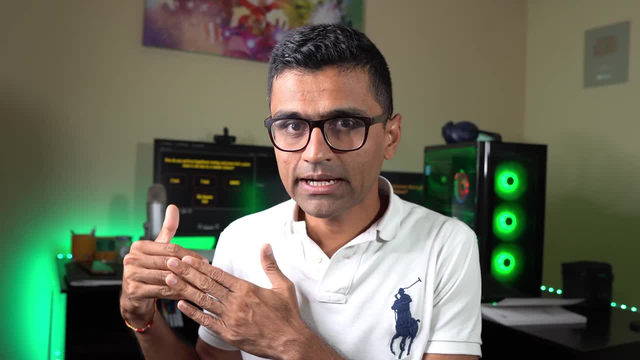 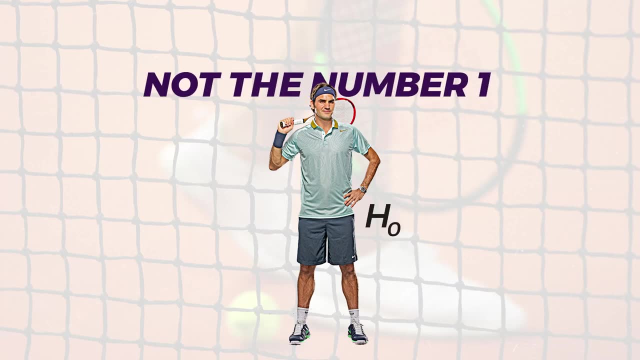 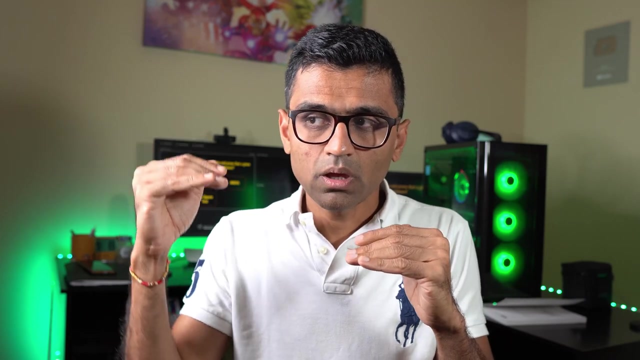 player than Federer. but instead of proving that, what if you prove that Federer is not the best Player or he's not the number one player, and when you do that, automatically number two- who is Djokovic- becomes number one. and you don't want to say that, okay, Djokovic is the best player because tomorrow 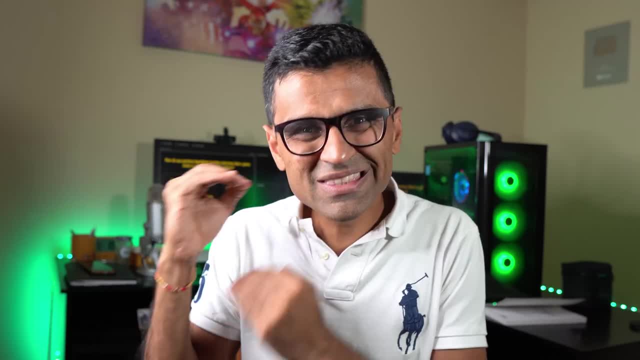 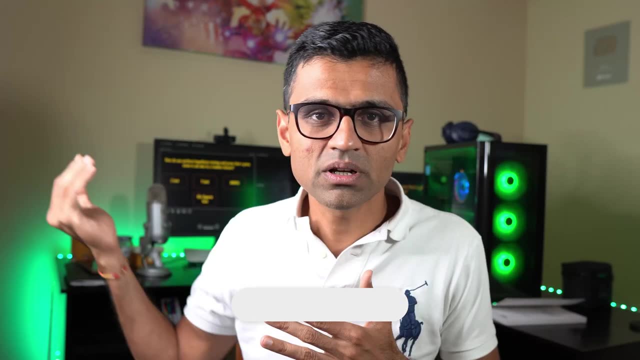 someone else might come in so that the statement that Djokovic is the best player, it's hard to prove. you know, it's not an absolute fact. things are always changing. so someone can come in and say: okay, someone, some new player will come and they, they, they can become a best player. so 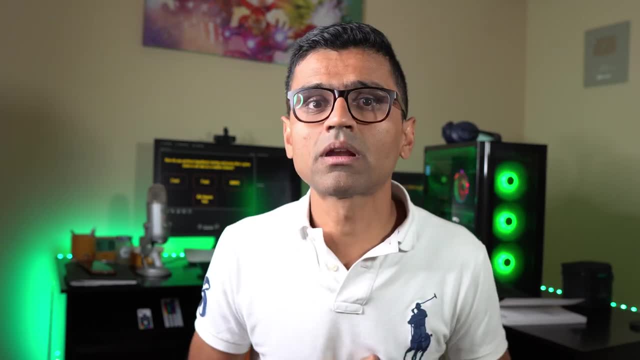 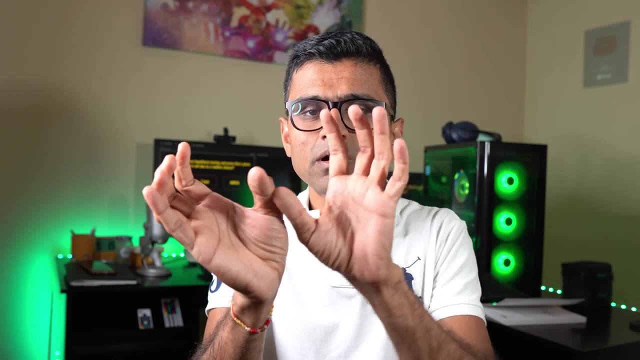 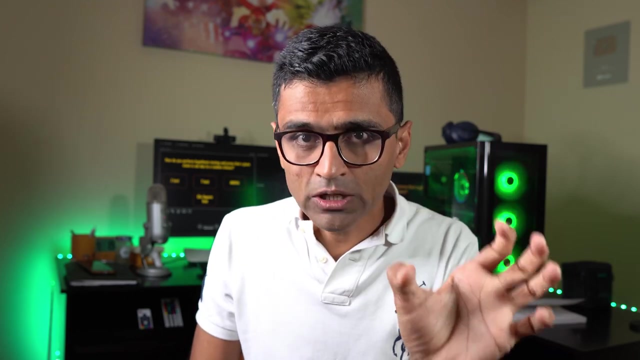 there's a whole idea behind having null hypothesis. so in hypothesis testing you have a claim that you want to prove. that is called alternate hypothesis. you go with the alternate claim, which is an which is an established fact or widely accepted phenomena, and you try to reject that. another example is: 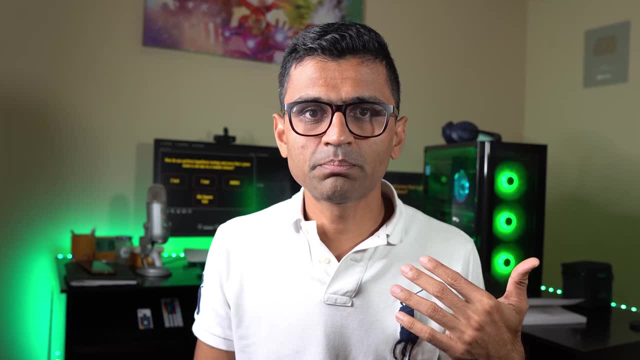 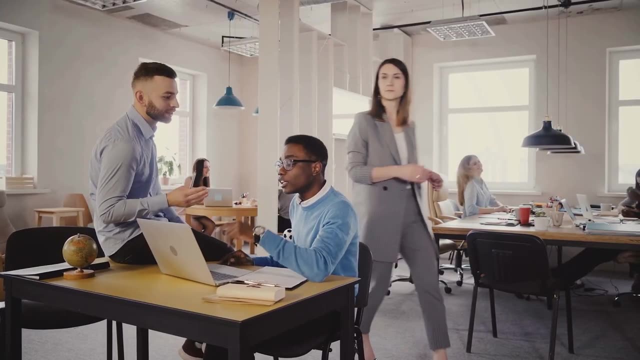 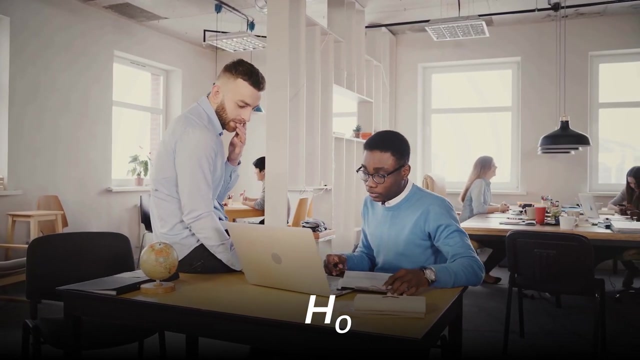 you know, up till now, before pandemic, the belief was employees are more productive in office. now that's how the world has been and everyone knows that. and you know that's my null hypothesis. and some HR people are coming up with a theory that employees can be more, can be productive at home also. so basically the opposite. 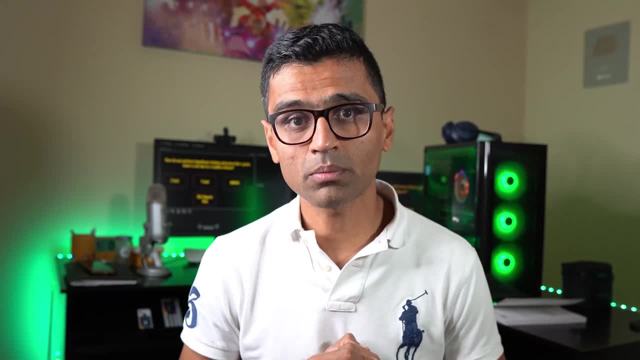 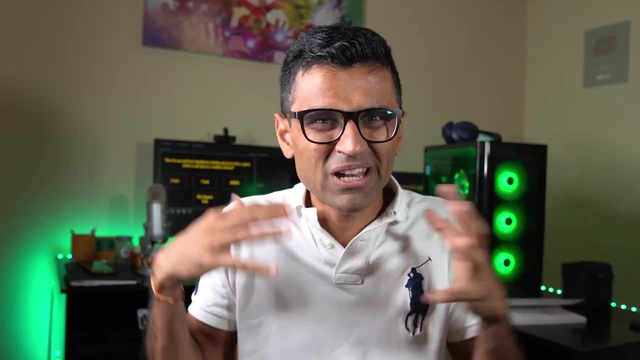 it's not like employees have to be in office in order to become more productive. now, that's a new thing. you know, that's a new thing. we have not experienced it much. maybe one and half year independent. now we know little bit, but people working from office has been like that since thousands of. 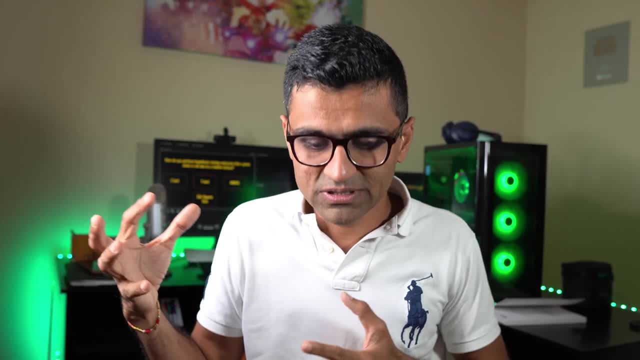 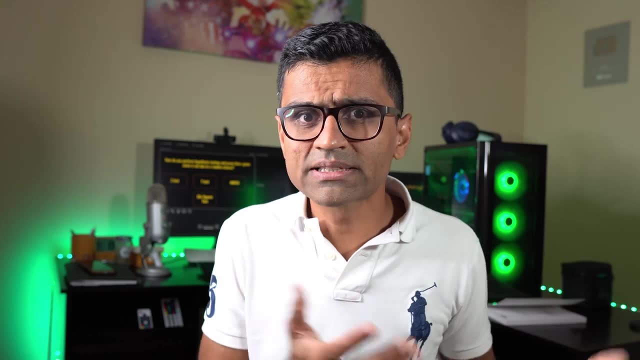 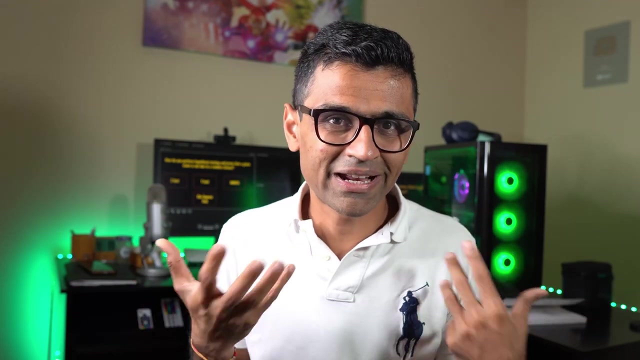 years. so that's my null hypothesis and my new hypothesis. alternate hypothesis is: employee can be more productive working from home as well. third example I want to give is irritable bowel disease has no relationship with food that you eat. that's an accepted belief right now in medical science. 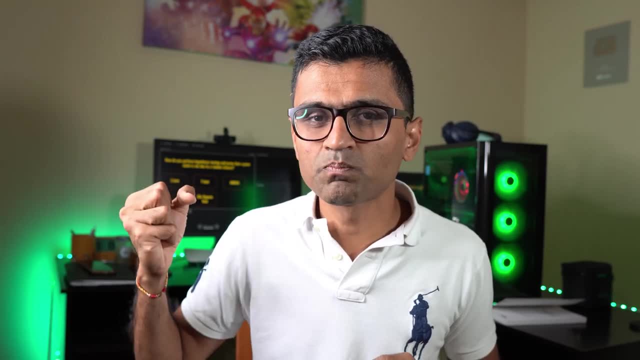 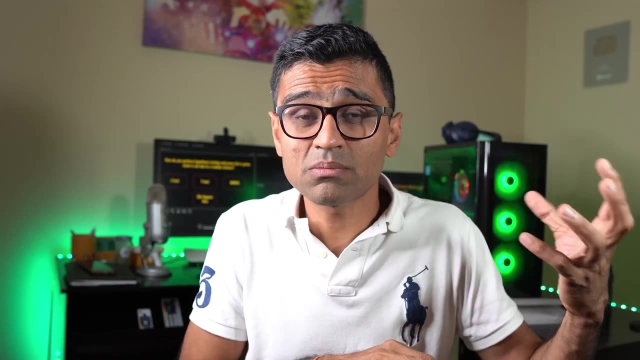 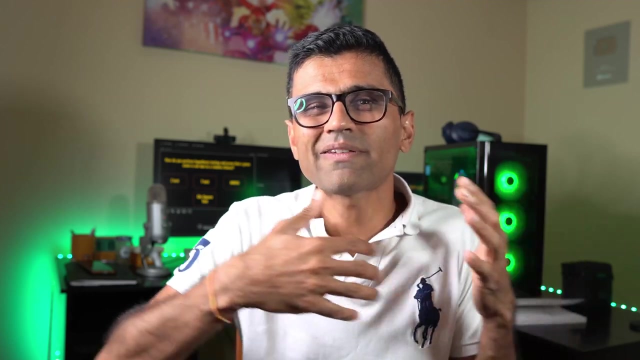 and some new scientists comes up with the theory that no, by eating certain food it can cause a irritable bowel disease. so then, the null hypothesis, which is irritable bowel disease has no relation with food. you can reject that. and if you reject that, you kind of establish the fact that